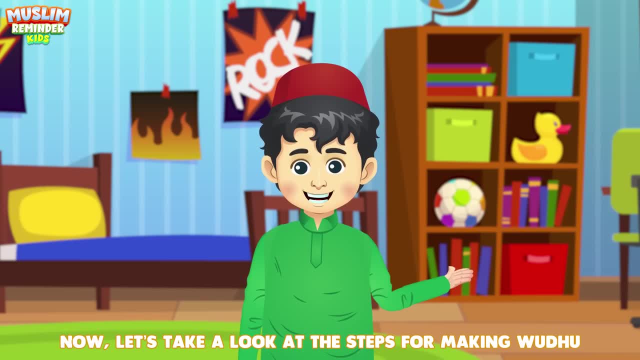 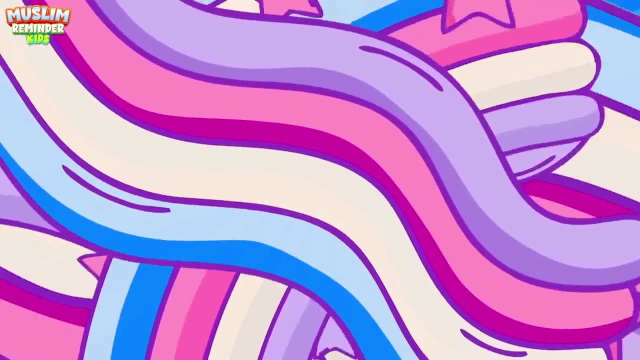 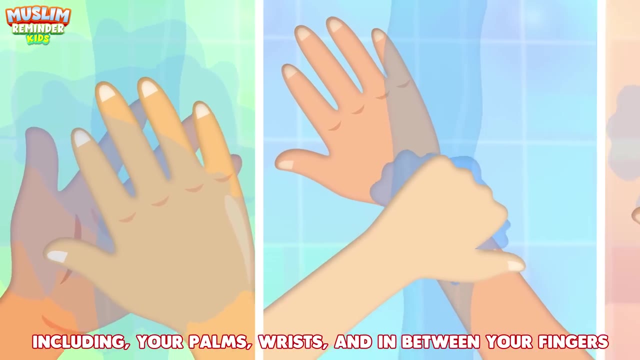 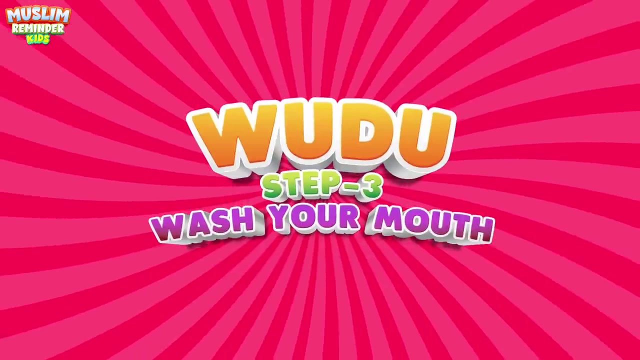 Now let's take a look at the steps for making wudu. Step one: You must start making wudu by saying bismillah. Step two: Wash both your hands completely, including your palms, wrist and in between your fingers. Repeat this step three times. Step three: Use your right hand to put some water into your mouth, Gurgle or rinse your mouth. 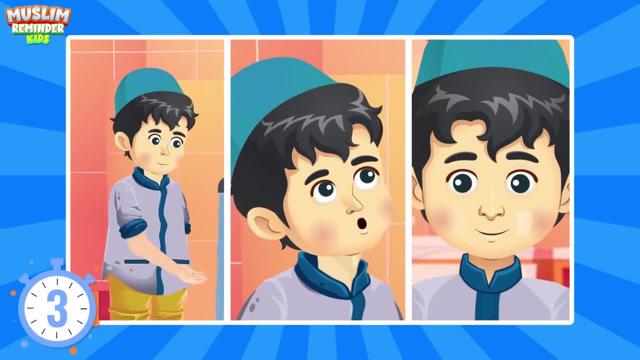 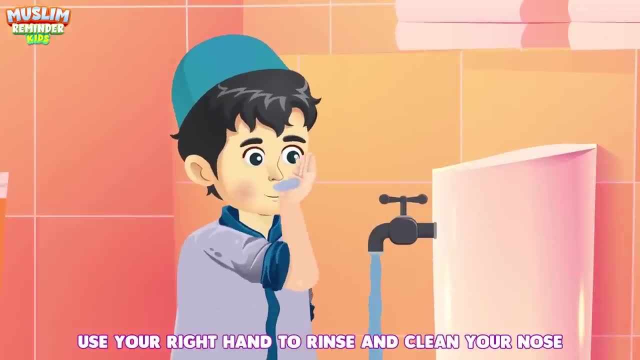 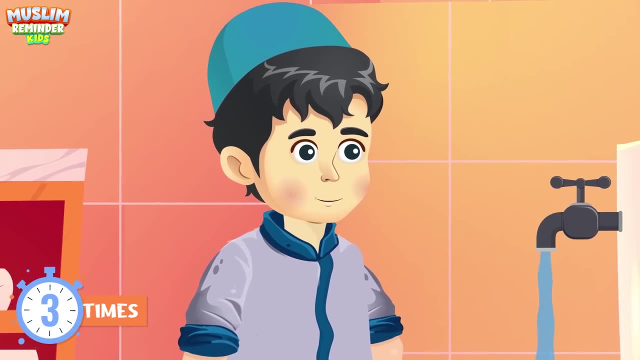 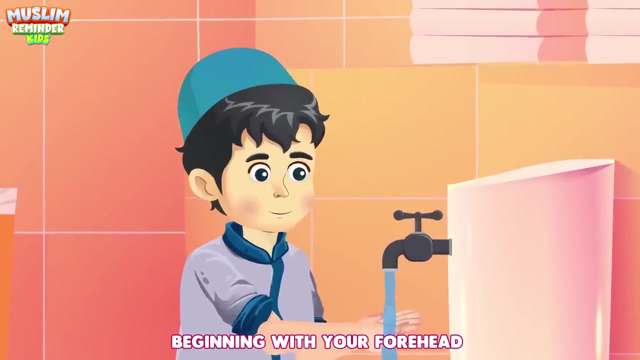 with the water and then spit it out. Repeat this step three times. Step four: Use your right hand to rinse and clean your nose by sniffing in some water, Then use your left hand to blow the water out. Repeat this step three times. Step five: Wash your entire face, beginning with your forehead and going down to your chin, and from your right ear to your left ear. 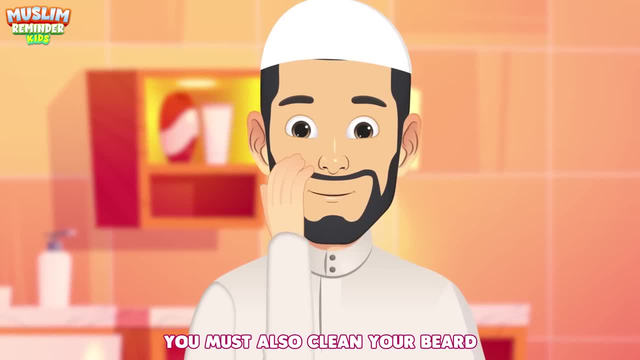 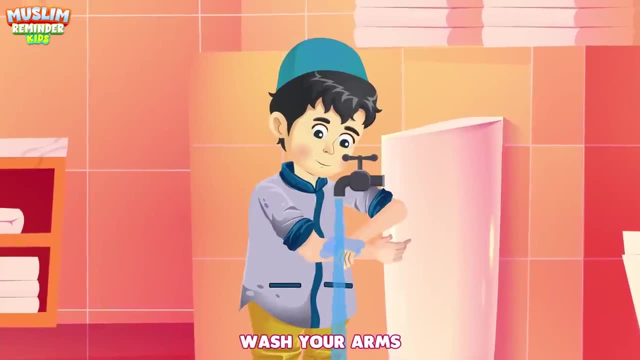 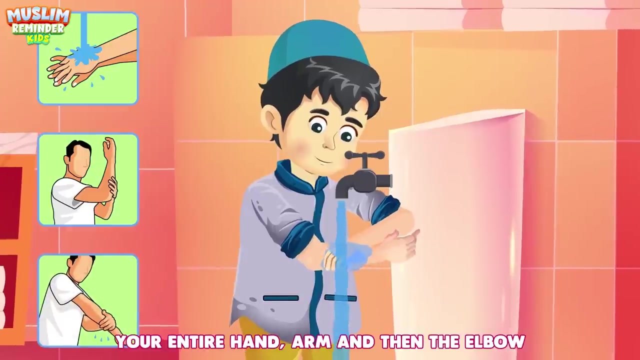 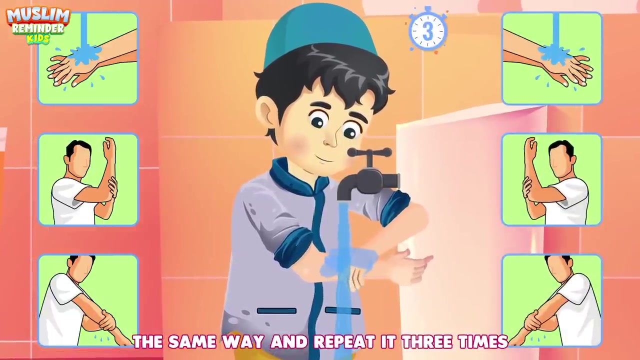 If you have a beard, you must also clean your beard. Run your wet fingers through the beard to clean it. Step six: Wash your arms. Begin washing your right arm, starting at the fingertips, your entire hand arm and then the elbow. Repeat this step three times. Then wash your left arm the same way and repeat it three times. Step seven: Wet your hands. 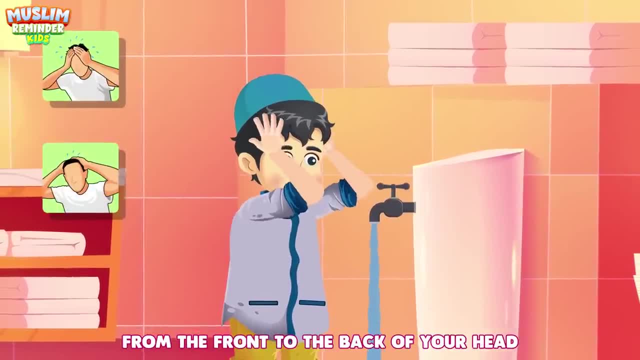 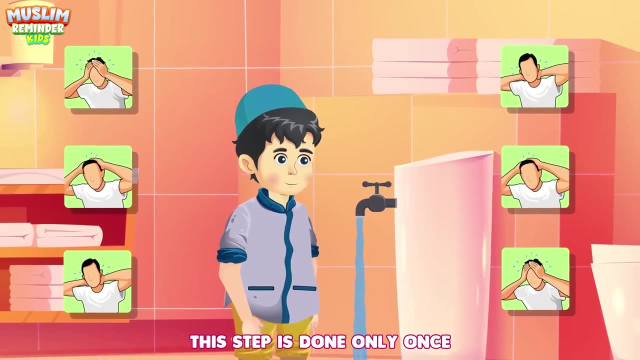 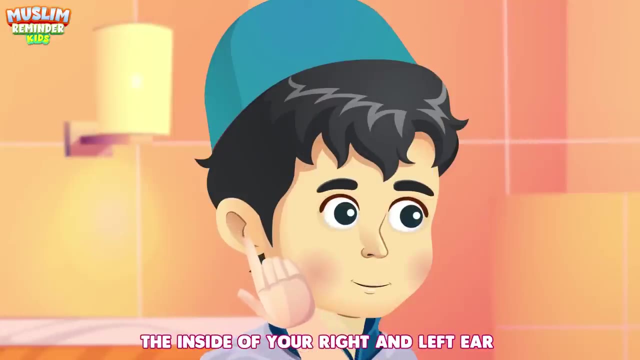 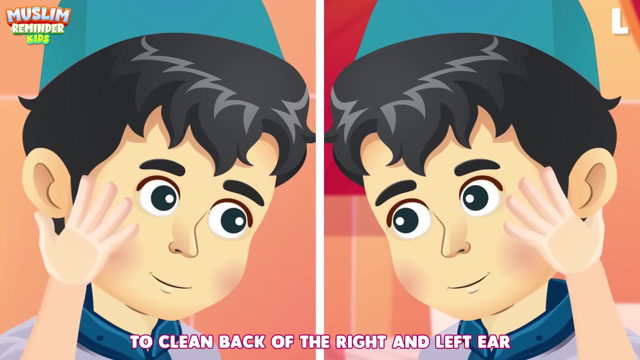 and wipe them through your head from the front to the back of your head and then back to front. This should be done in one move. This step is done only once. Step eight: Use your index finger to clean the inside of your right and left ear to remove any dirt. Then use your thumb to clean back to the right and left ear. This step is done only once. Step nine: 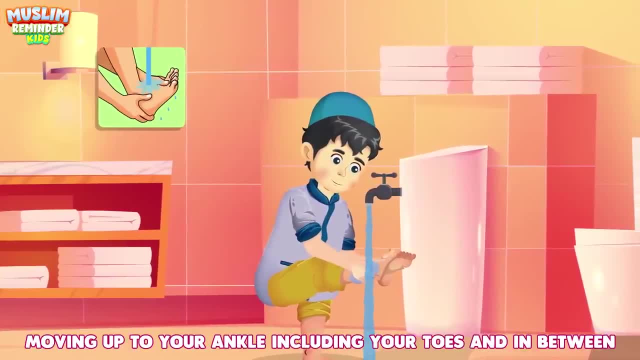 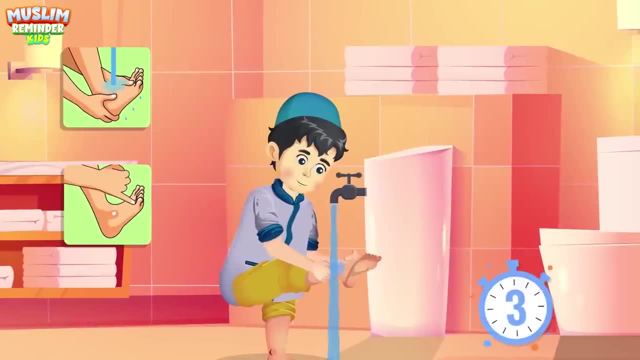 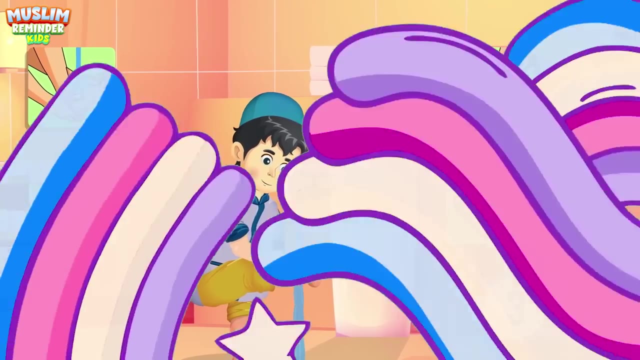 Wash your right foot, moving up to your ankle, including your toes, and in between Use your pinky finger to clean in between your toes. This step must be repeated three times. Then follow the same steps for your left foot and repeat it three times. Step ten: